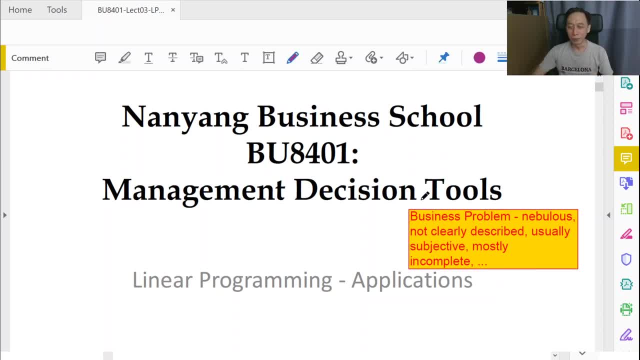 not clearly or fully defined. So let me put a kind of a cloud around it, just to suggest that this situation is kind of not even easy to describe, not to mention to solve it right. So to solve it means to select a choice, to make a decision such that certain thing is: 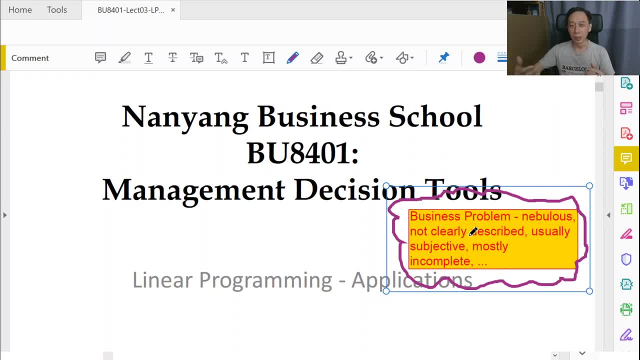 certain measurement by certain count. it is the best, it is optimal, And we learn about that. the equivalent of it in linear programming model will be the objective function, And objective function is a mathematical expression that links into the decision variables right, So the decision variables will be the. 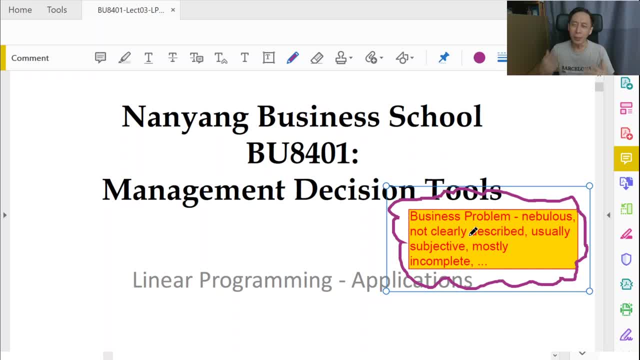 hmm, I wonder how many or what, how much should certain amount, certain business variable be, so that I can maximize it? So let's say that I have a business problem and I have a business problem and I want to minimize my profit or minimize my waste, yeah, So these are the cloudy situation. 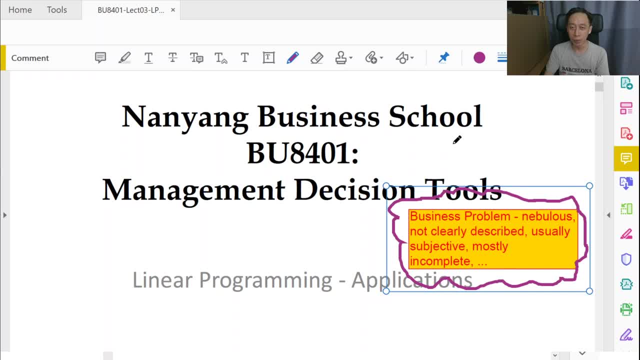 that we wish to translate. So our job is to translate into a very clean, clear and well-defined mathematical decision description called the model right. So we want to have a mathematical model And in our case, we're going to use the LP model um. 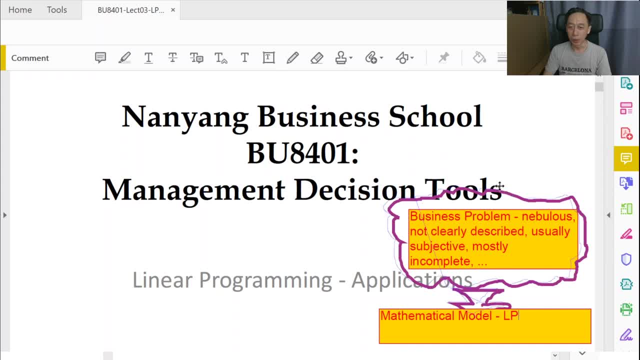 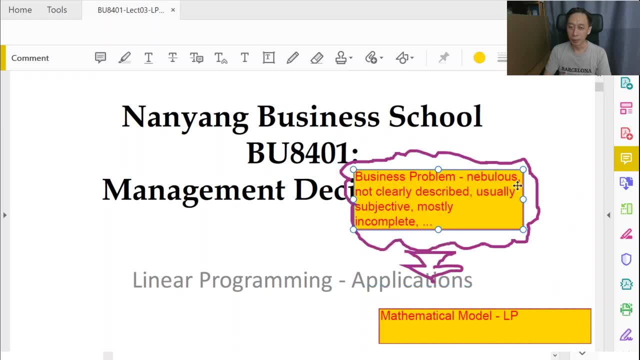 to describe what we are interested in. Okay, so, so let me also move this up. Yep, okay, So the process of trying to um solve a particular situation will involved first, as a first step, a translation into mathematical model, or, you know, as a 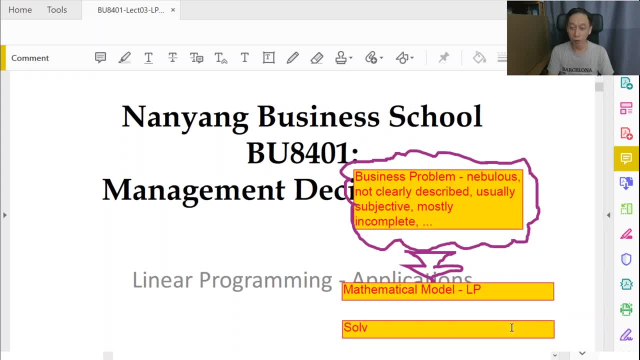 LP model. And the second step then is to solve the LP model, say using Excel solver. that's one way, And the reason why we split it into two steps is because the first step involves a translation kind of skill. that is, we appreciate the situation, we look at the parameters, 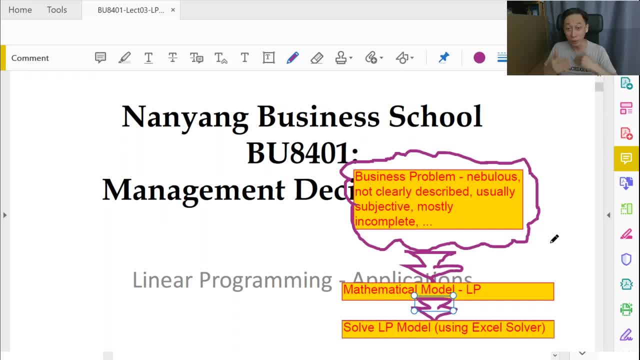 we look at the interrelationships. If it's non-linear, we try to approximate it, justify it correctly with mathematical theories or our domain knowledge and understanding of the business, so as to say that, well, this linear approximation is as good as the non-linear. 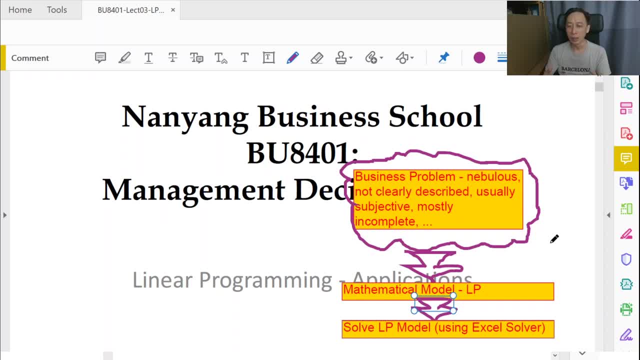 behavior in real life, So as to arrive at a clean-cut, well-defined and completely defined linear programming model. So that's our first stage, right, our first step Now, once we are at this step, a lot of expertise can come in right computers can come in. 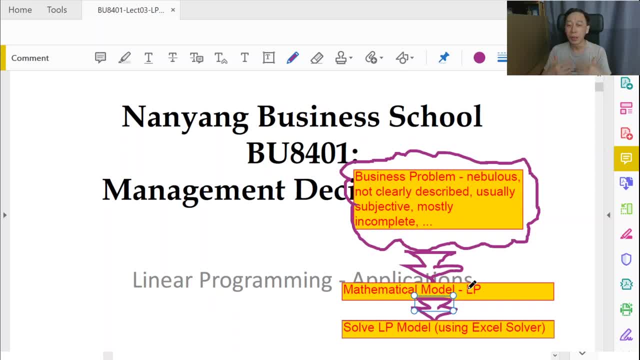 software can come in, packages can come in, consultants can come in to try to solve for the numerical solution. So there are two steps involved, And so should you be thinking about that in applying linear programming models in your project, exercises, exams or at real 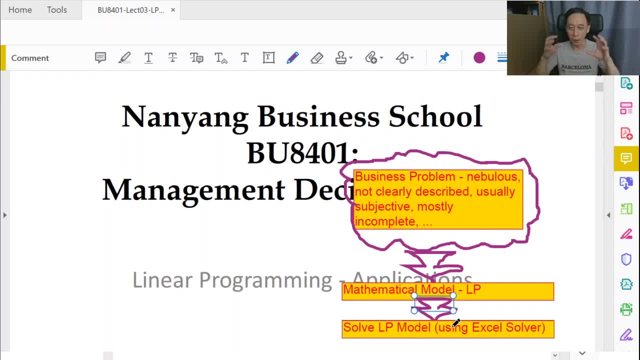 life, work and projects. So in this particular session we will focus mostly, in fact only on the first step. The first step is the most challenging step, the most value-adding step and the step that is perhaps kind of too unseriously. 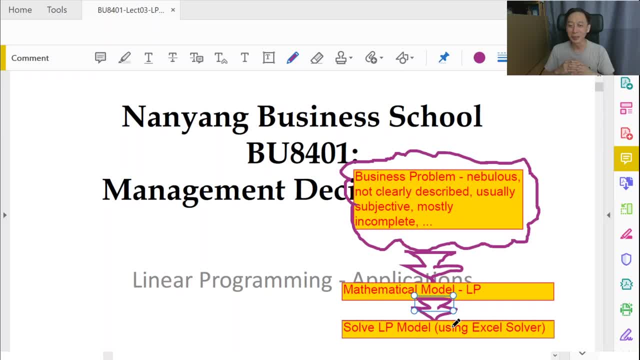 ignored by most beginning students. learning this, That is, you don't get a solution after the first step, The output is a mathematical description. There is no answer, no numbers as the result. So the sense of completion and perhaps academic satisfaction doesn't seem to be there. But 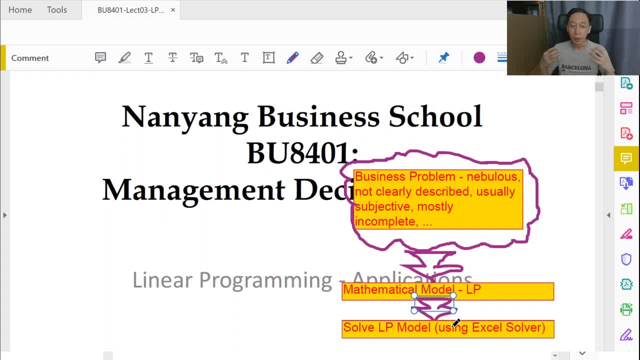 it is the most value-adding step in terms of actual real-life working scenario, because you have just made a very hard problem- invisible problem, not clearly visible problem- right in this cloud into a very clean-cut, well-defined mathematical solution. 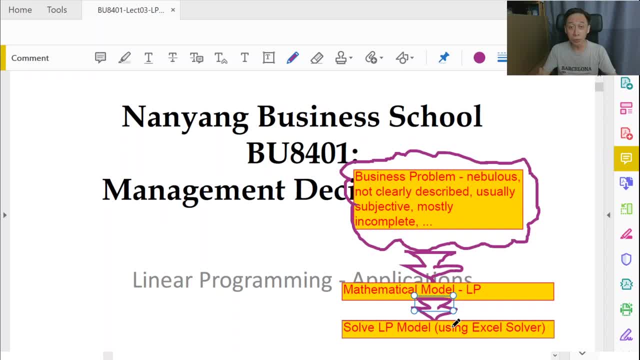 So this is the first step. So we are having a very complex model. The first step is to work through this model, which can be understood by a lot more people beyond the business owner, beyond the business manager involved in the original problem, right? 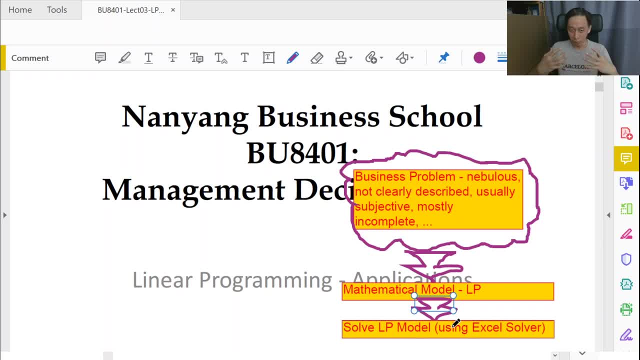 So this value-adding step is what we will discuss more, because there are tricks and skills involved in trying to come up with the model And, in particular, the constraints Right. So this is the first step. So after a few exercises you will begin to get a hang of it so as to be able to solve most problems. Of course, difficult ones still arise, but we will try to empower you with the commonly encountered situations. 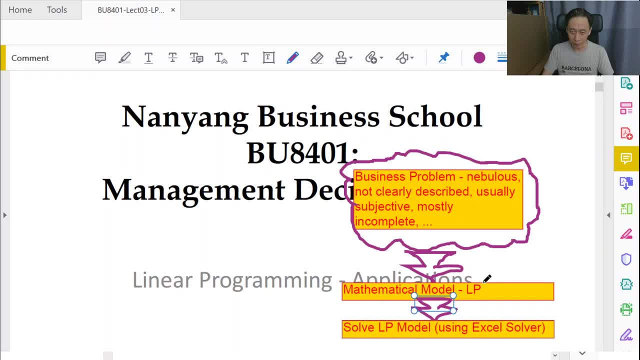 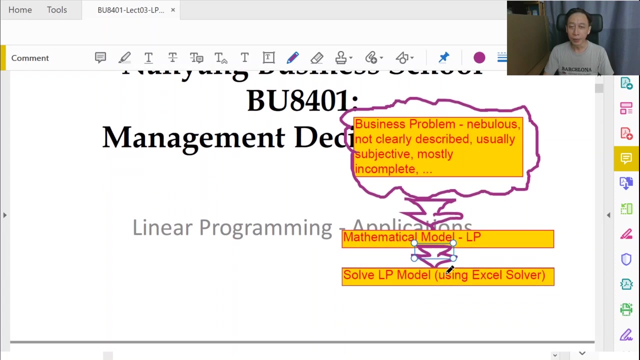 And once we are able to do that then it is rather easy to apply solver packages- Python, R, MATLAB, Mathematical and whatever packages you like to go from the LP model, Mathematical model, to get the actual numerical solutions. So in this session we will examine three examples taken from the LP model. 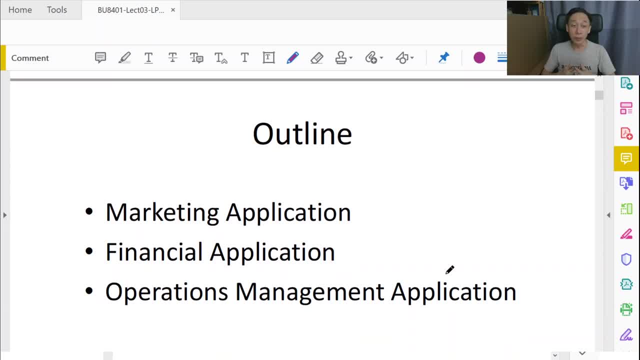 Intentionally three different industries and applications. But other than changing the story, changing the terminologies used, right instead of saying eyeballs, exposure in marketing to returns and interest rates in finance, Other than just changing the words, we will also learn different tricks along the way. 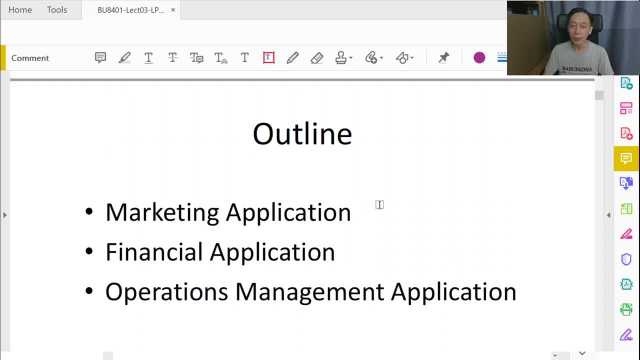 So, in particular In the marketing application that we will discuss, we will learn how to identify such constraints as proportionate constraints. What are proportionate constraints? How do they behave? You know things like that- Proportionate. So we'll learn about proportionate constraints here. 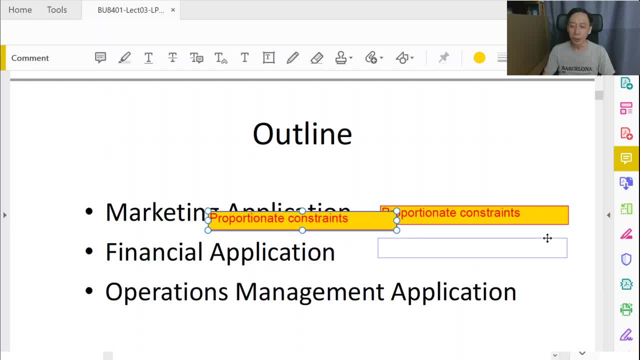 Then we will learn about how to improve, how to implement or describe time- Right time in LP. How do we do that? How does time get represented in the LP model? And, lastly, we learn through the example. in operations management. We'll learn how to identify. 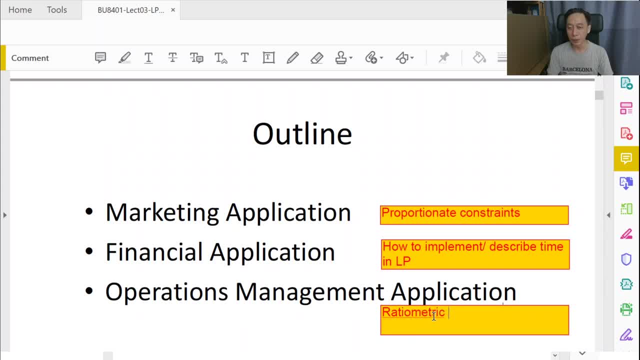 ratio, metric constraints And, at the same time, how to implement or describe leftovers Or access or surplus, as in the surplus that we described, learn about in previous video sessions. so that will be the those rather map, more model oriented aspects rather than business oriented aspects. 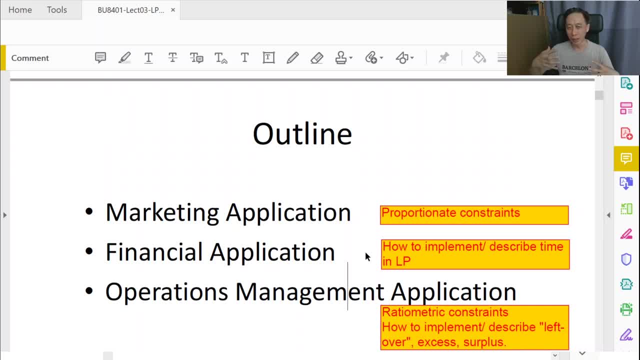 of how we might appreciate they are. they are being they, that they are being used in real life. so what will trigger, for example, a situation in which we write down a proportionate constraint, a ratio, metric constraint, if we have a situation involving time, hey, which business application. 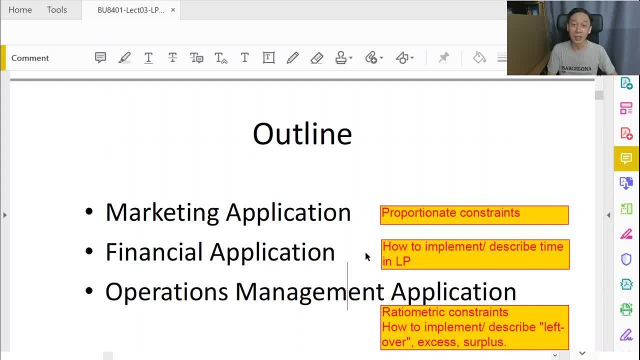 doesn't involve time right. so very commonly we'll encounter time. and how do we implement time? because in lp model the sequence, the order of the constraints doesn't indicate before and after. so writing a constraint first does not mean that time, whether in real time or otherwise. 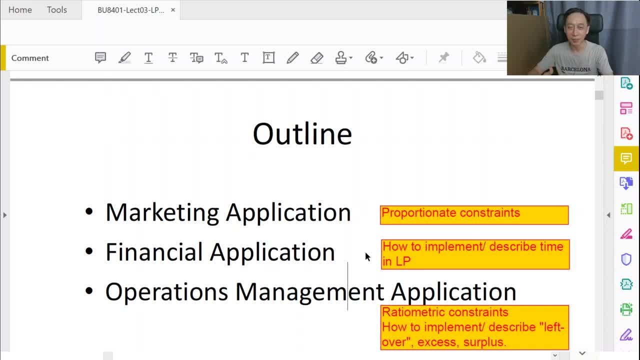 that constraint is bound first or is being satisfied first. there's no such thing. so how do we tell our lp model that this has to be satisfied first, before that? you know how do we tell time, all right, so? so that's one trick, and very important trick that we have to learn. 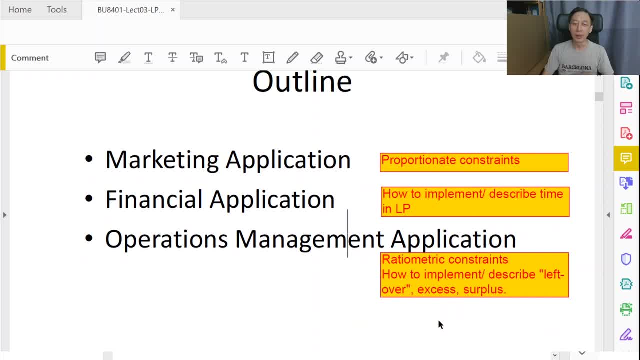 and finally we learn about situations, about ratio, metric, uh- constraints. what are they and how do they sound like in real life? we might learn the mathematical expression, but you know there's a it. it appears differently if you are the consultant trying to identify it. without anyone hinting you. that is a ratio metric constraint. how do you smell that? how do you?